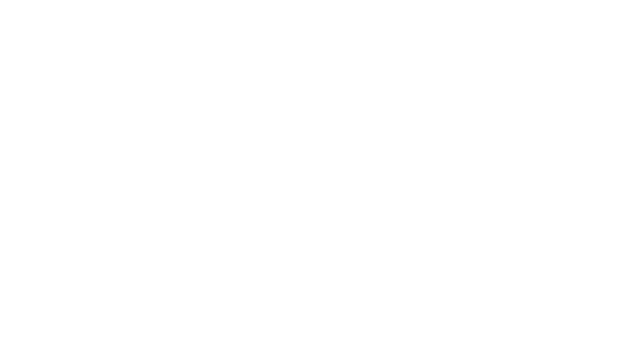 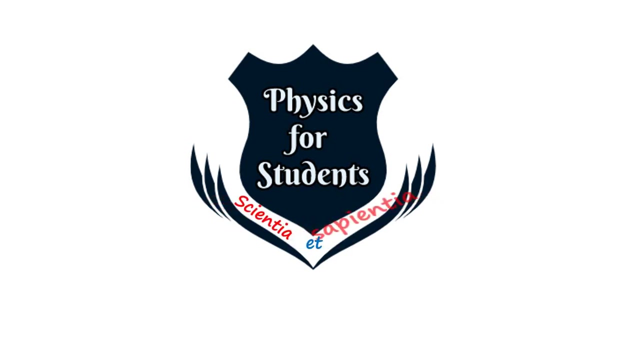 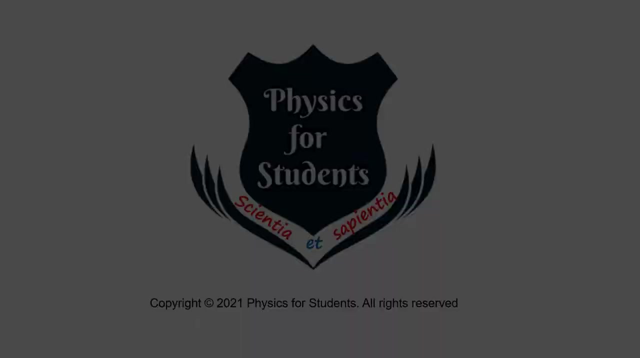 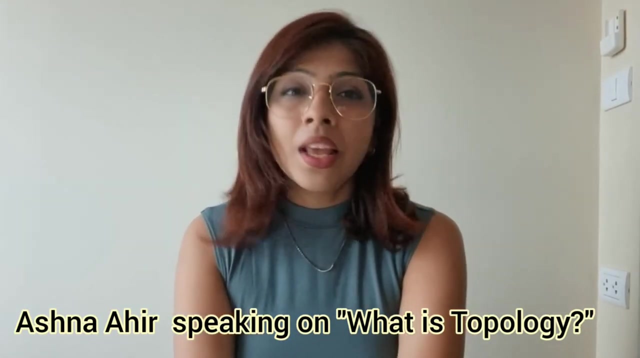 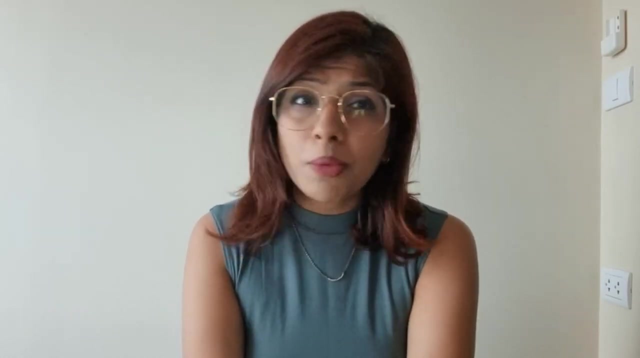 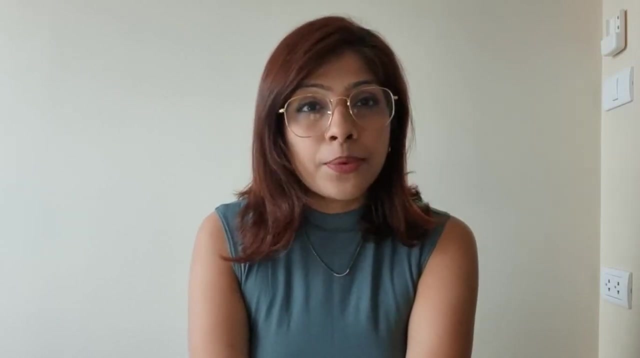 Hi everyone. my name is Ashna and I'm a TEFL Certified English teacher. Have you guys ever wondered that a coffee cup and donut is the same? That's crazy, right, Or maybe not? Topology is the branch of mathematics which is also called rubber shaped geometry. It deals with 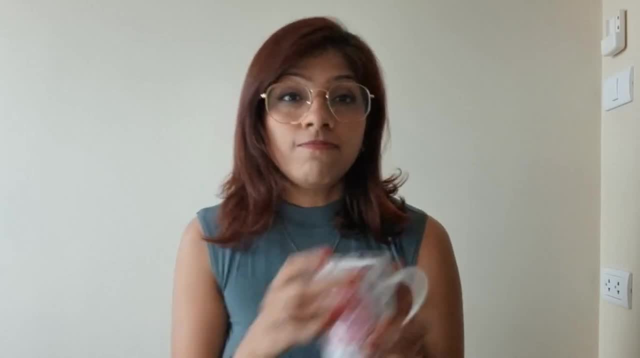 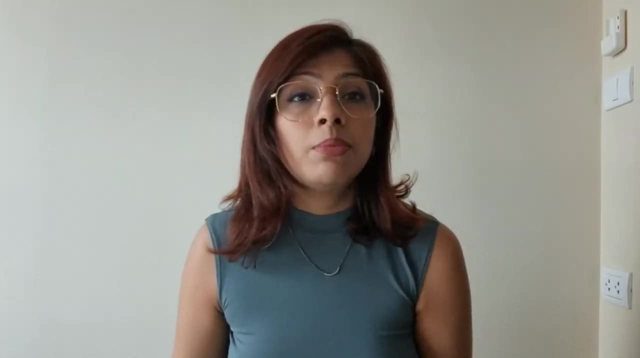 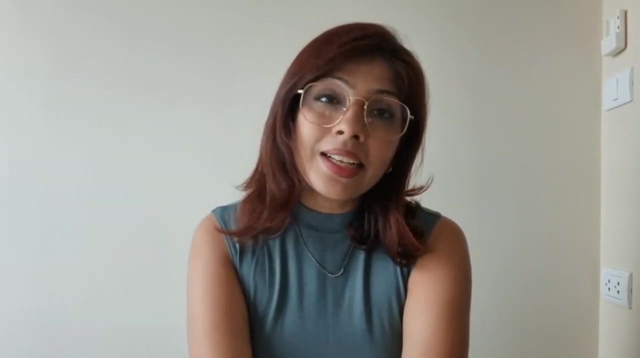 different shapes and sizes. It may deal with this cup or it may deal with this circular shaped platter. Basically, all these shapes can be turned, twisted or stretched. Topology basically deals with all shapes and analyzes their different forms. The advantage is that 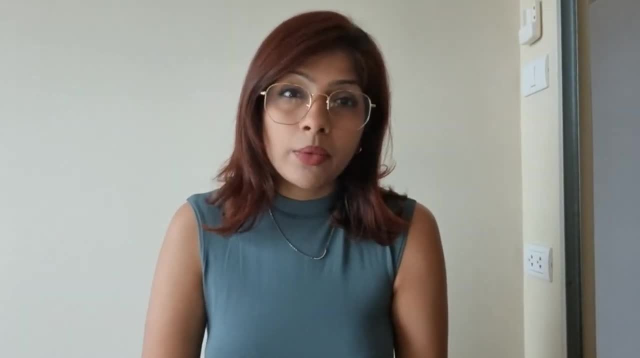 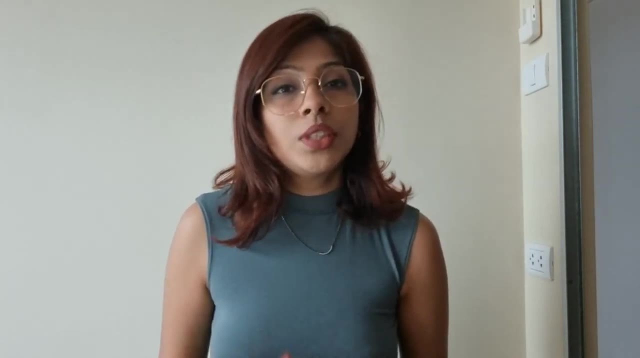 when we deal with Euclidean geometry, we create a formula by which we can say that if a particular shape, for example a square, equals to a rectangle, then we can also say that the properties of the square also equal to the properties of the rectangle. Topology carries the same formula. 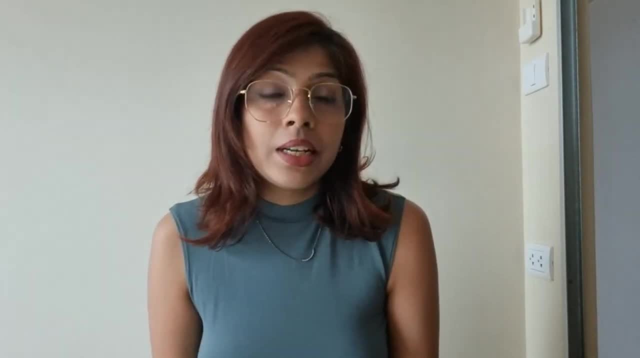 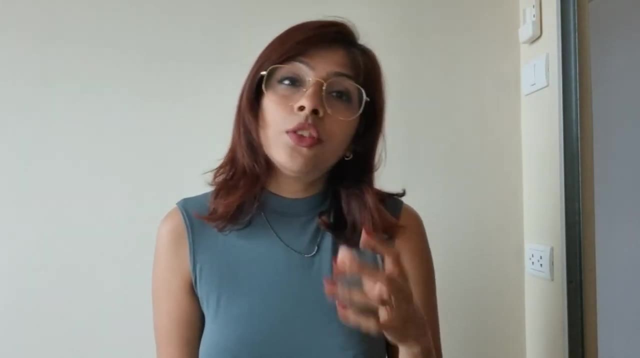 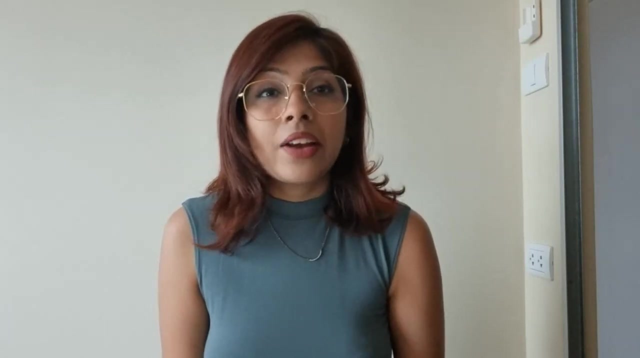 and the same feature and can deal with any object, Maybe a cup, a sphere, a rectangle or any other object. So, basically, if we know the features of a particular shape and even though it is deformed and turned into another shape, it will still carry the same features. 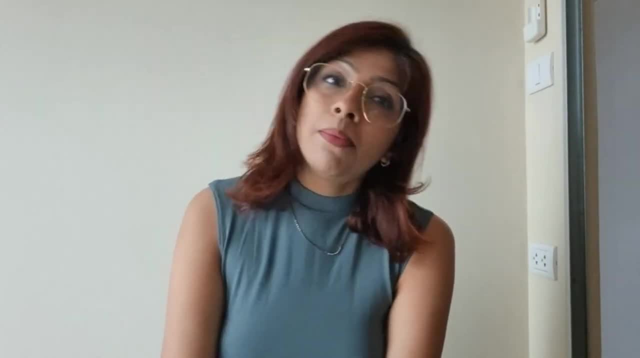 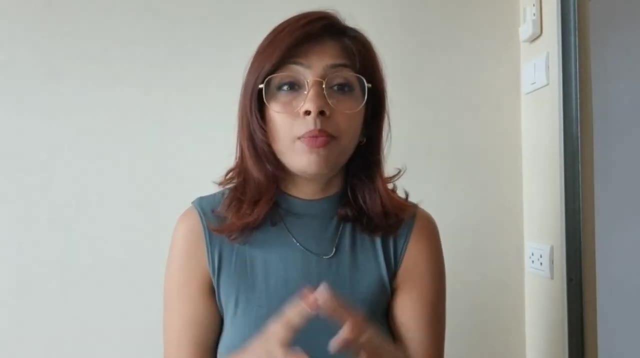 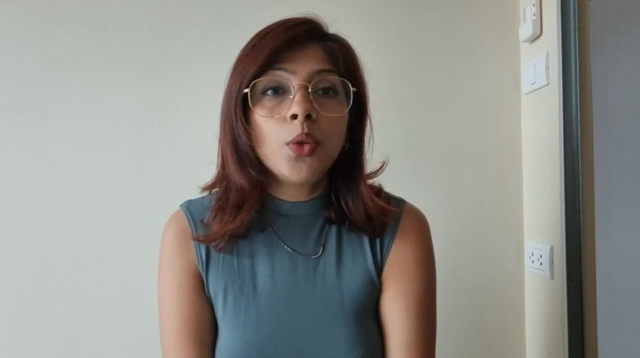 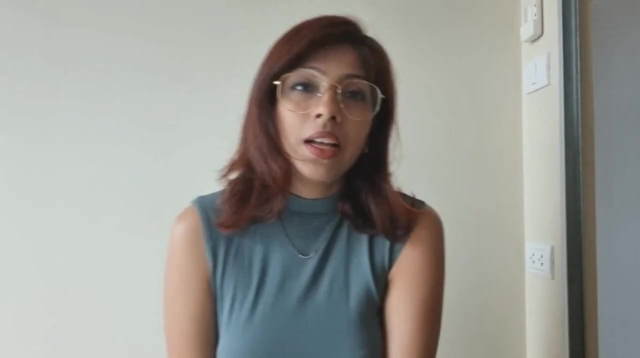 The motivating insight behind topology is that many geometric problems depend not on the exact shape of the objects involved, but rather on the shape of the object itself. Topology is the foundation of geometry. Topology is the foundation of geometry. Topology is each two larger. объ 1983, First discourse: Topology and geometry work. 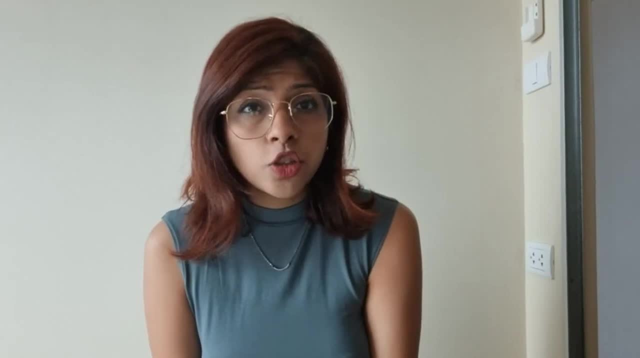 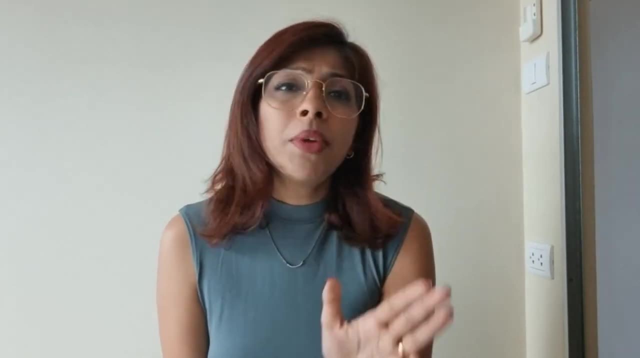 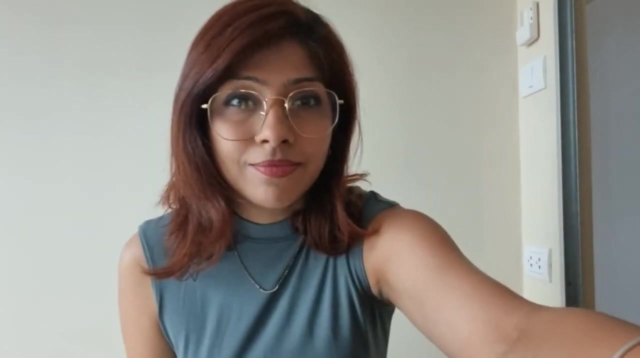 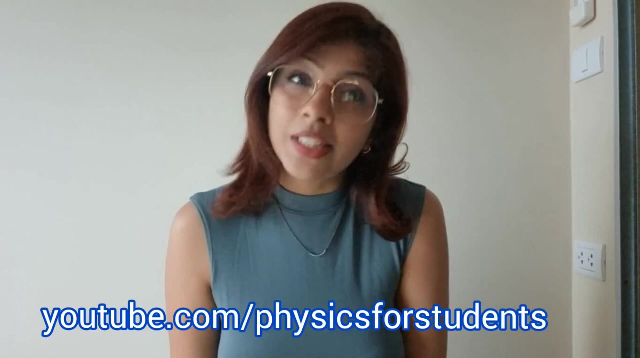 length. Topology has many different branches, liked algebraic topology, general topology, differential topology, geometric topology, etc. We should not be confused by the wahrscheinlich different. We are talking about mathematical topology. If you're interested in the topic of topology, I would highly recommend you to check out the channel Physics for Students.